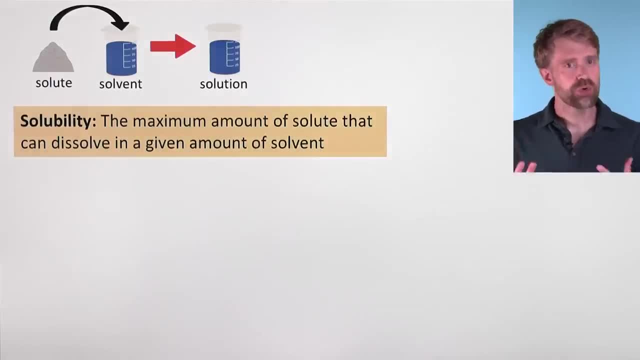 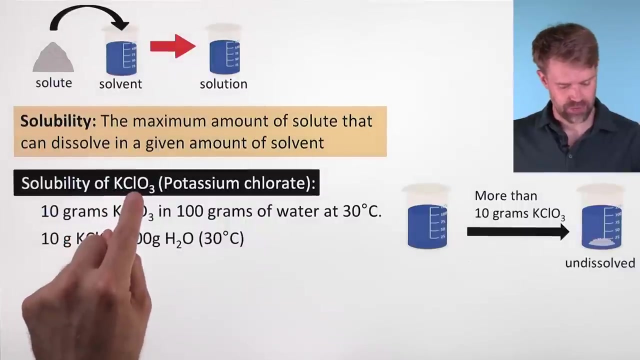 is called the solution. Now, a super important concept with dissolving is solubility. Solubility is the maximum amount of solute that can dissolve in a given amount of solvent. So, for example, we could look at KClO3 potassium chlorine and its solubility is 10 grams. 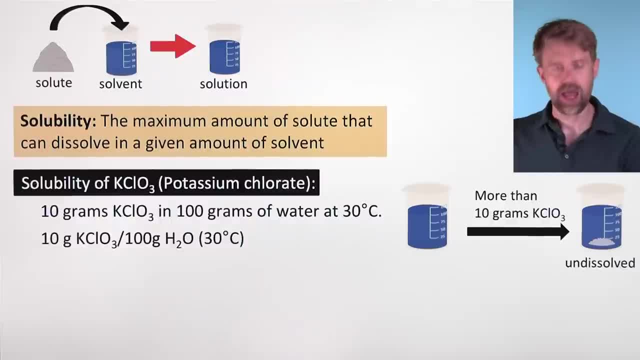 KClO3.. ClO3 in 100 grams of water at 30 degrees Celsius, So more than 10 grams of potassium chlorate, and it's not going to dissolve. It'll just end up on the bottom of the container. Now notice that I. 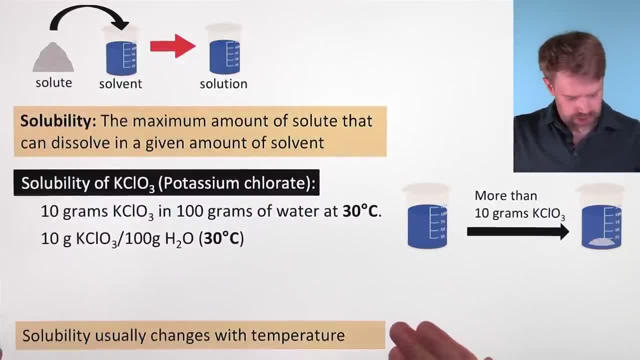 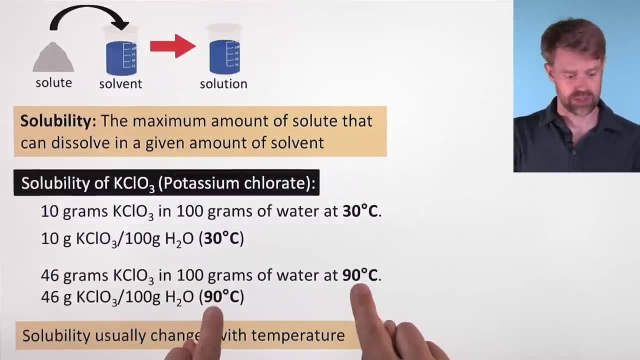 said 30 degrees here, and that's because solubility usually changes with temperature. For example, at 90 degrees Celsius, 46 grams of potassium chlorate can dissolve in 100 grams of water. That's pretty different. Now, since solubility changes with temperature, it's often convenient. 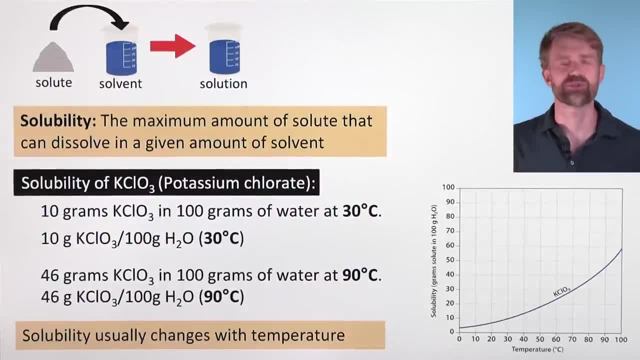 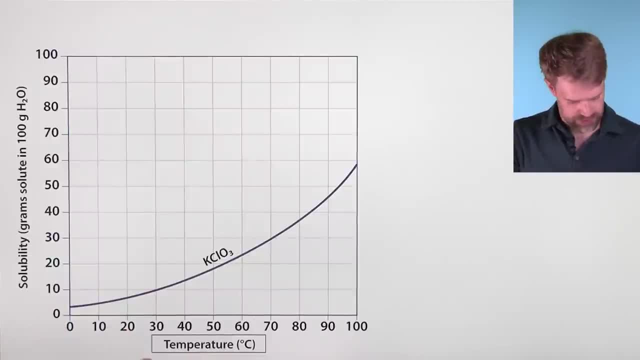 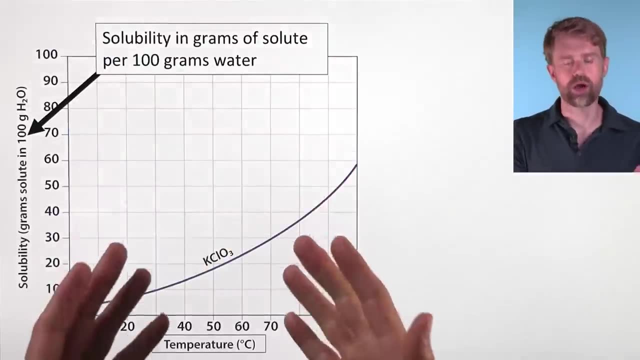 to show this on a graph. Let's take a closer look Here. on the x-axis we have temperature in degrees Celsius and on the y-axis is solubility- Solubility in grams of solute per 100 grams of water- And obviously this line here shows us the 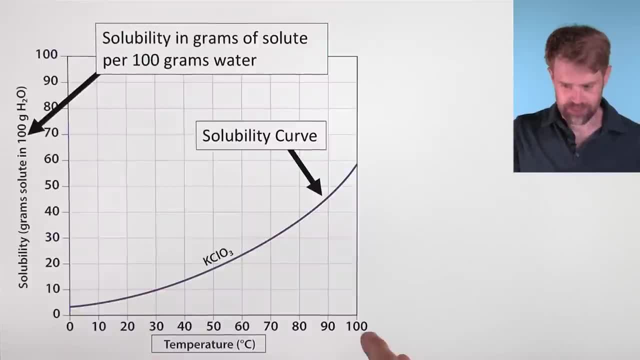 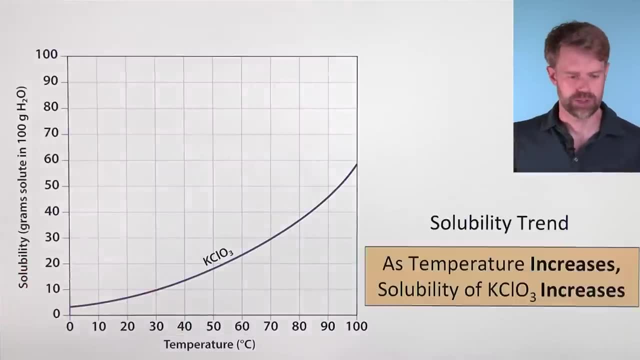 solubility of KClO3 at different temperatures. We call this line the solubility curve, And this type of graph is useful in a bunch of ways. First, we can quickly see a trend For KClO3, as temperature. 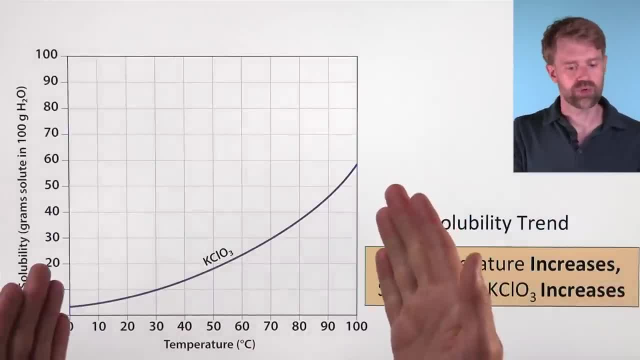 increases, the solubility of KClO3 increases, So we can quickly see a trend For KClO3,. as temperature increases, the solubility of KClO3 increases, So we can quickly see a trend. So there's the. 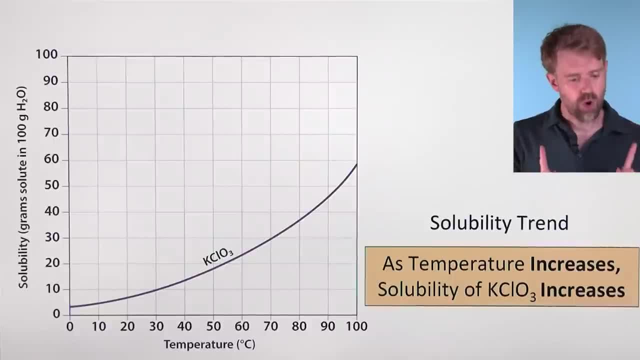 new graph we're looking at. Okay, so that's important. That's one thing that we can see right away. We can also use the solubility curve to get specific numbers for solubility and temperature in different situations. Here's an example. 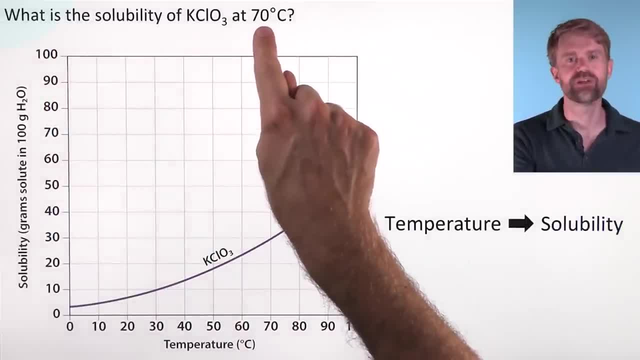 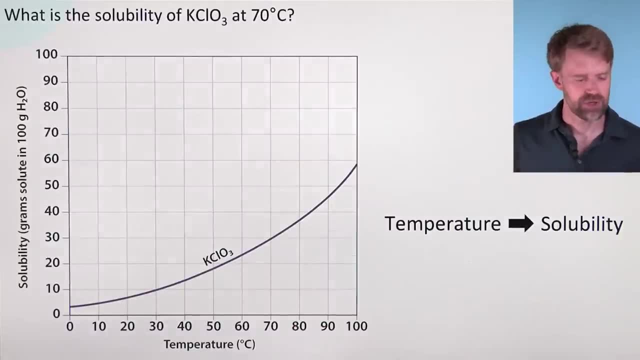 What's the solubility of KClO3 at 70 degrees Celsius? It gives us a temperature and we want to know the solubility at that temperature. Here's what we do. We find 70 degrees on the x-axis. 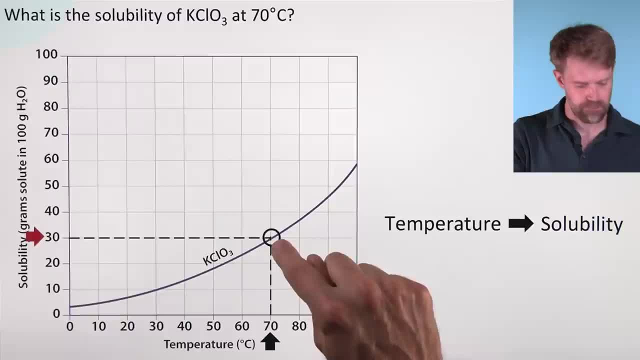 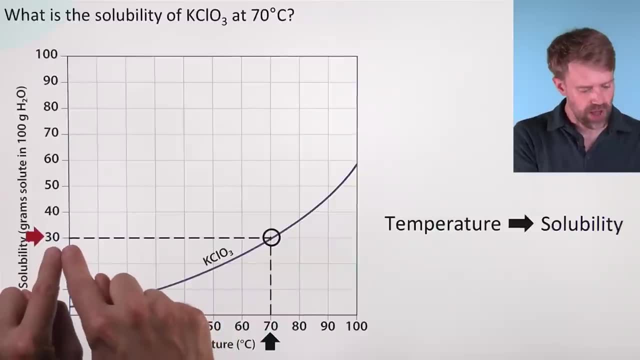 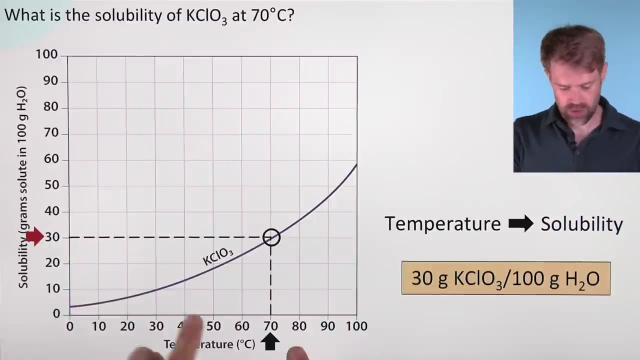 We go up to the solubility curve and then we go across and we look at the y-value for solubility. We find the y-value where it intersects And here that looks pretty much like 30. So the solubility at 70 degrees is 30 grams of KClO3 per 100 grams of water. 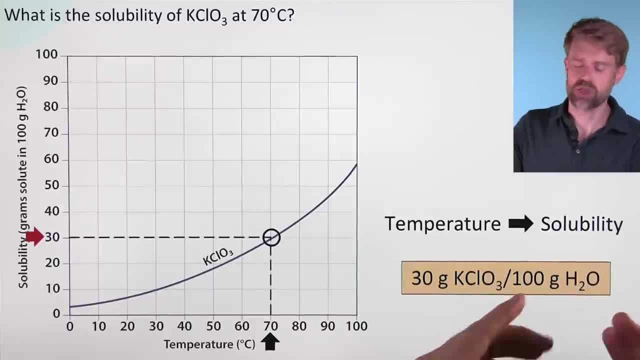 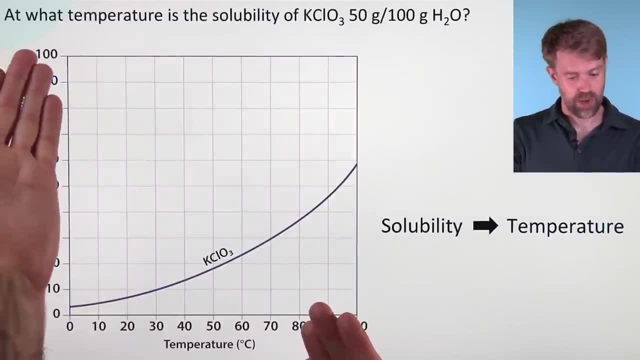 Remember that solubility is per a certain amount of solvent. It's usually 100 grams of water. when you're looking at curves like this, Now we can also go the other way. At what temperature is the solubility of KClO3?? 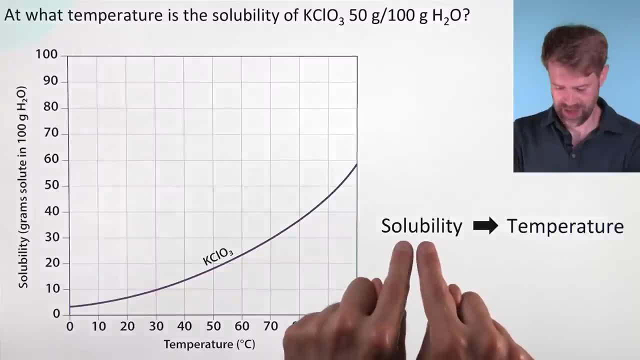 50 grams per 100 grams of water. Here we have a known solubility. We want to find the solubility, We want to find out the temperature where we have that solubility. So we'll do the reverse of what we did previously. 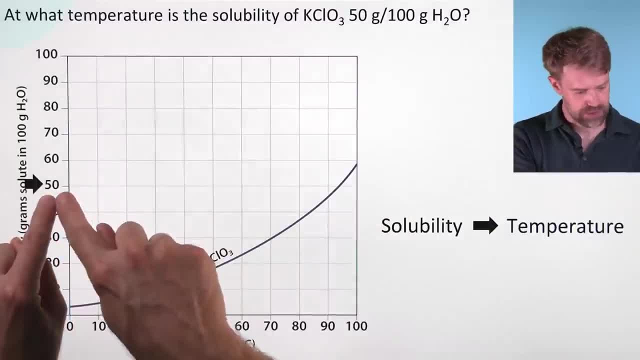 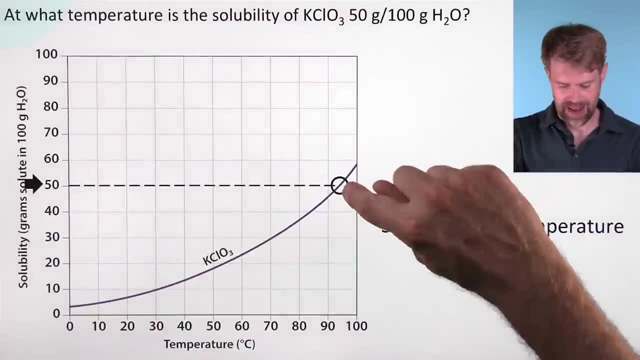 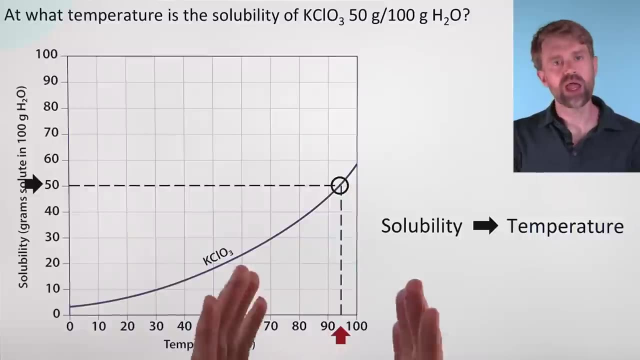 We go to the y-axis and we find 50 grams per 100 grams of water. We go across until we intersect with the solubility curve And then we go straight down until we hit the x-axis. Now, this isn't right on a number, so it's going to require a little bit of estimation. 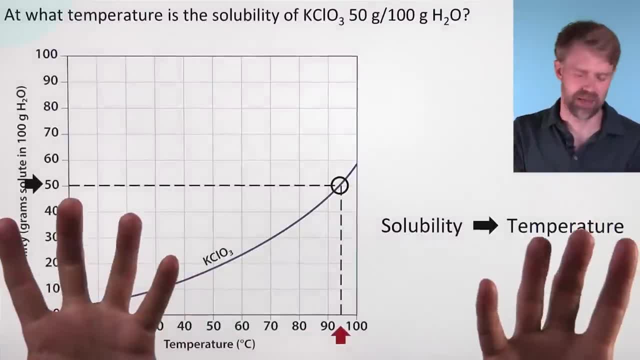 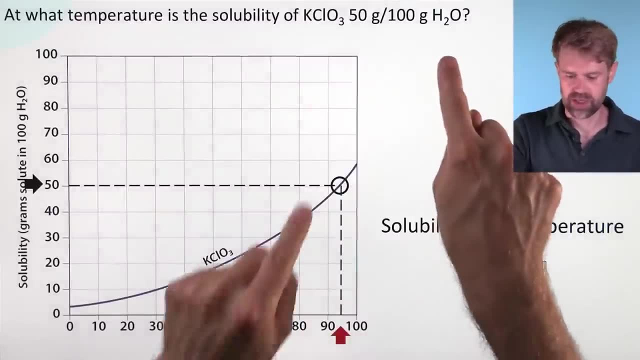 We know it's going to be 90.. We know it's going to be 90.. We know it's going to be 90.. The final digit is going to be our best guess. So let's say 95 degrees, And that's the temperature where the solubility is 50 grams per 100 grams of water. 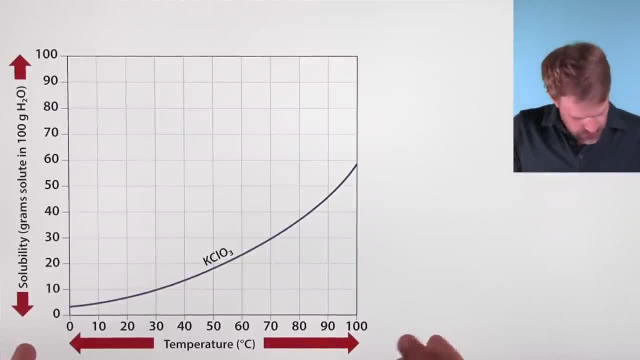 So, as you can see, we can find temperature and solubility information for all the points on this curve. Now, obviously, this curve shows us the solubility for just KClO3.. But usually when you see solubility curves, 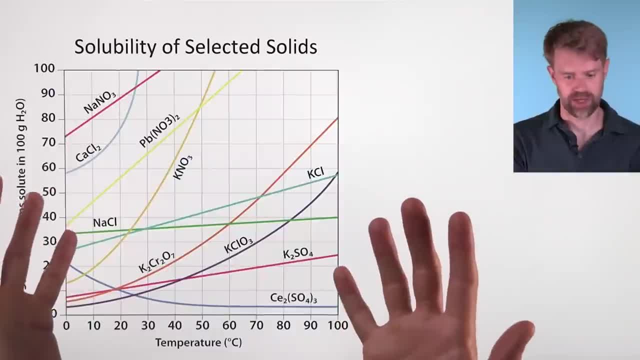 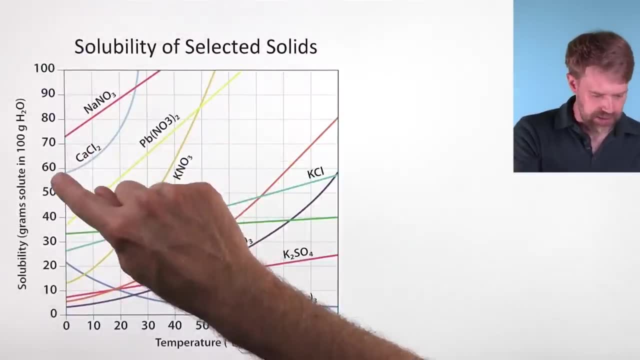 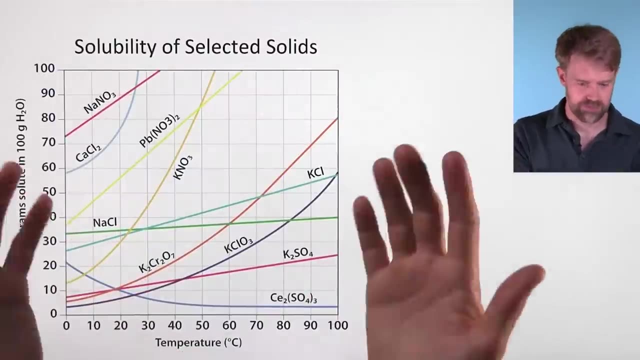 they'll be on a graph with lots of others like this. All these lines represent different solutes. We've got sodium nitrate, calcium chloride and all these others. They all have different solubilities. We often put them on the same graph so that we can save space. 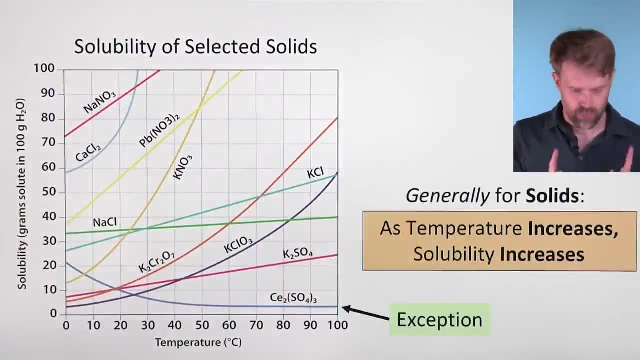 but also so that we can compare them And right away we can see a general trend. These are all solids And generally, as temperature increases, the solubility will increase. Solubility increases as well. There are some exceptions, like cerium sulfate here, that becomes less soluble with increasing temperature. 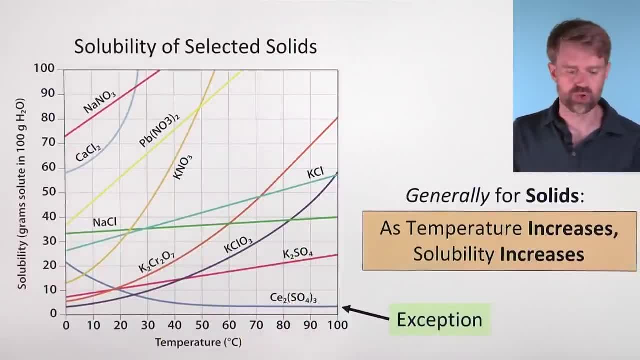 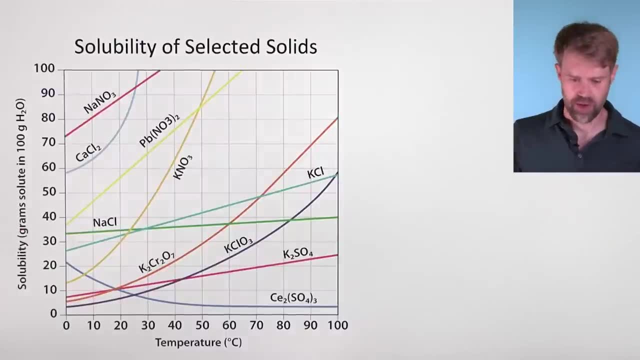 But generally solids are going to follow this important trend. Now, all these lines, all these different solutes can look confusing on one graph, But luckily you can just focus on the curves that you need to answer a specific problem, Pretend the others aren't even there. 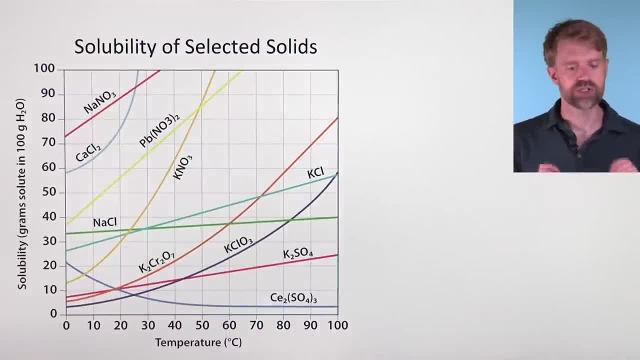 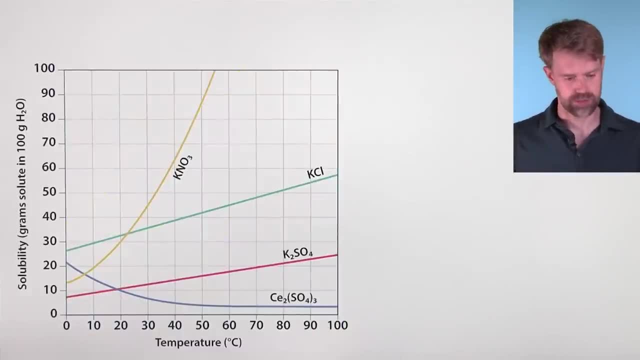 For example, the practice problems that we are going to do here are just going to focus on four different solutes. So boom, we can ignore all the other lines And we'll start off with two problems that use only the curve for potassium chloride or KCl. 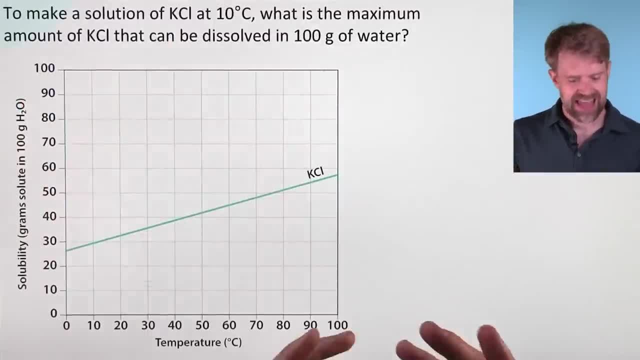 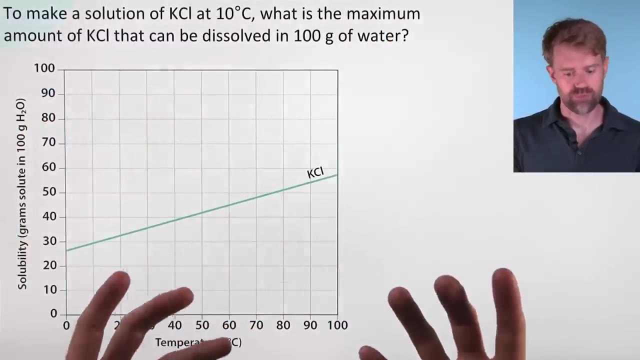 To make a solution of KCl at 10 degrees Celsius. what's the maximum amount of KCl that can be dissolved in 100 grams of water? We're looking for the maximum amount of KCl, So it sounds like we're looking for the solubility. 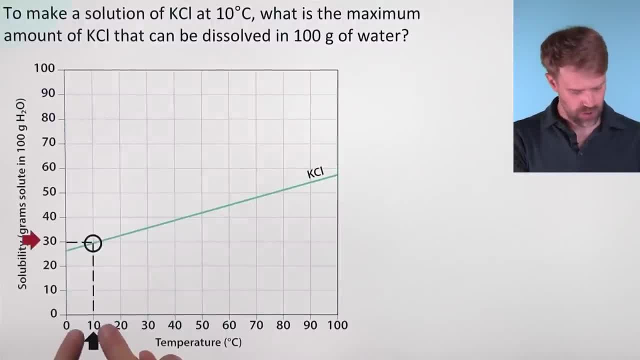 in 100 grams of water. So, as we did before, we start at 10 degrees Celsius, go up to the curve across to the Y-axis and we get 30 grams. 30 grams can dissolve in 100 grams of water. 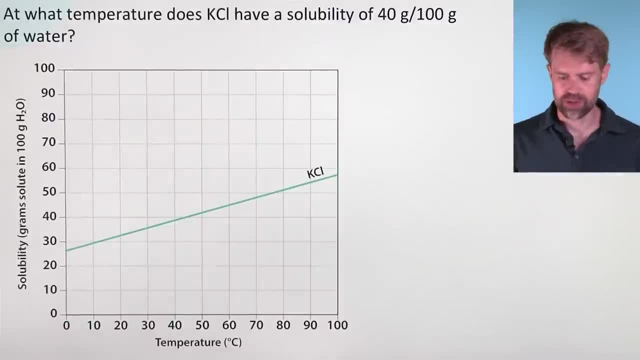 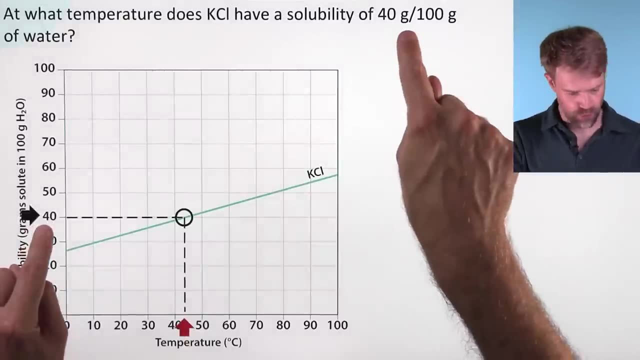 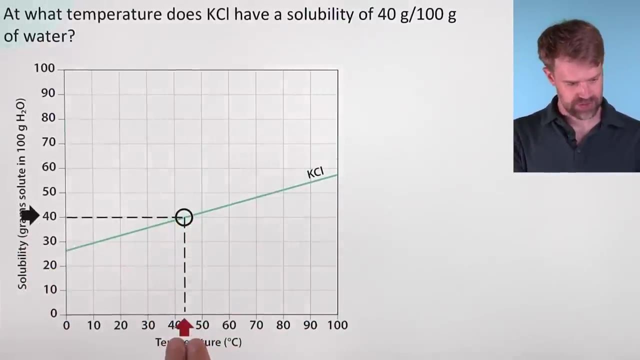 At what temperature does KCl have a solubility of 40 grams per 100 grams of water. Okay, we start at 40 grams per 100 grams of water on the Y-axis, across to the solubility curve and down to the X-axis. 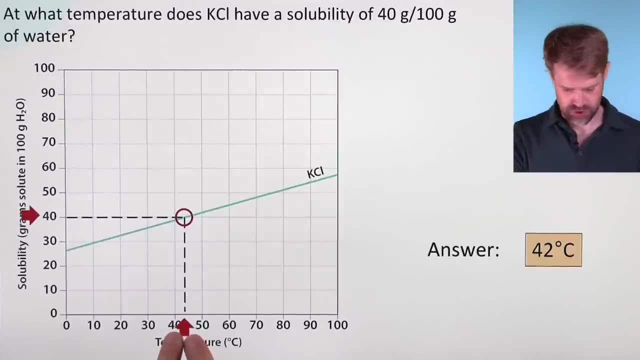 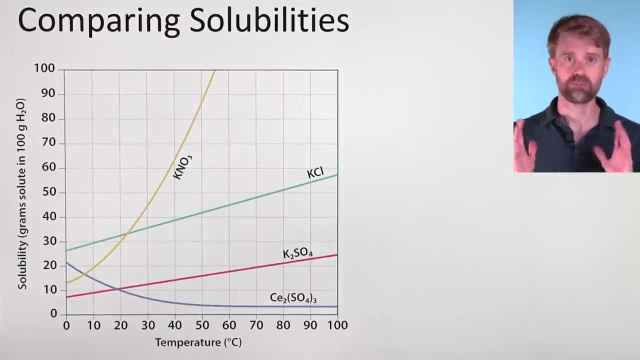 It's gonna be 40, something we've got to estimate, let's say 42.. 42 degrees Celsius is the temperature where KCl has that solubility. Now, as we said before, graphs like this are really useful for comparison. 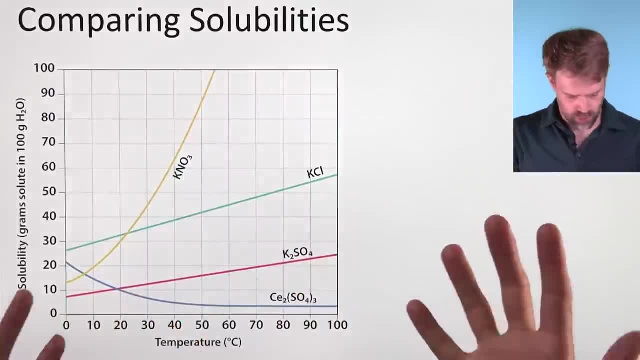 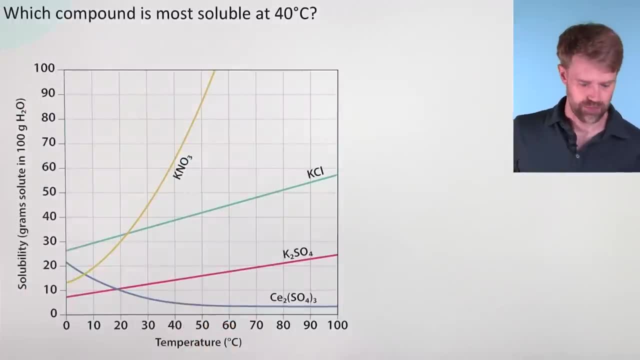 We're comparing solubilities between different solutes. So here we'll bring back some curves for the other solutes and we'll ask which compound is most soluble at 40 degrees Celsius. So first off, we find 40 degrees here on the X-axis. 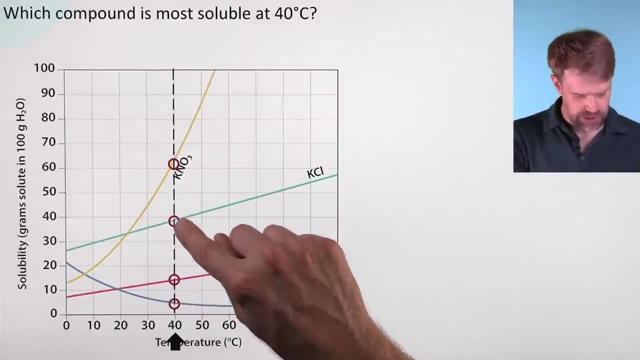 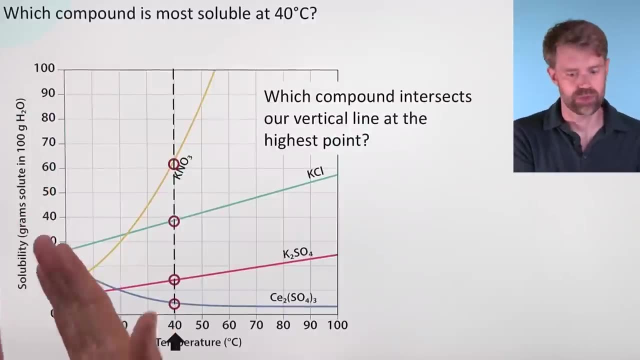 we draw a vertical line and we'll see that it intersects each one of our curves at one point. And to find the most soluble compound, we don't even have to worry about the specific values on the Y-axis. We just need to find which compound intersects this line. 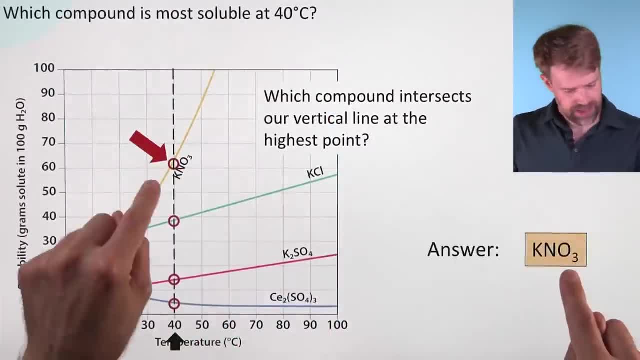 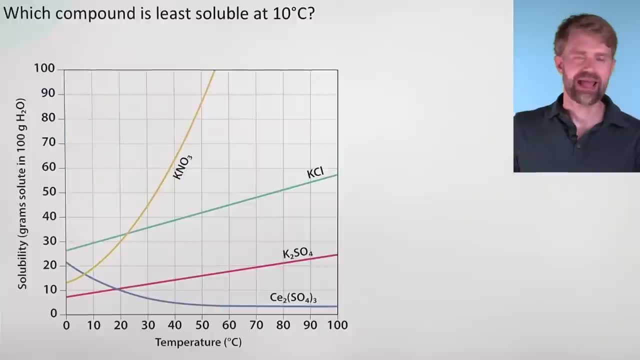 at 40 degrees at the highest point, And clearly that is KNO3, potassium nitrate, That is the most soluble at 40 degrees. We can ask a similar problem but, flipped around, Which compound is least soluble at 10 degrees Celsius? 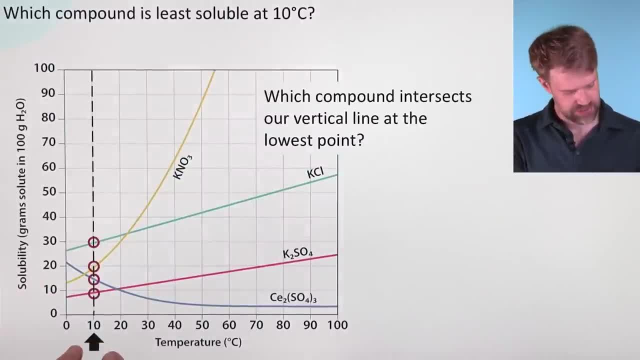 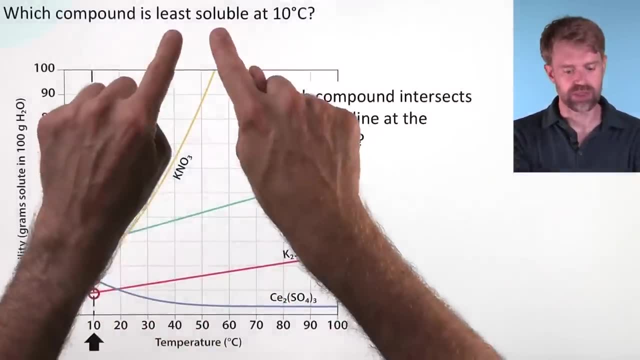 We're gonna do the same thing: 10 degrees Celsius on the X-axis. there it is Vertical line up, boom, boom, boom, boom. four intersection points, and this in this case, since we're looking for the least soluble compound, we're gonna ask: 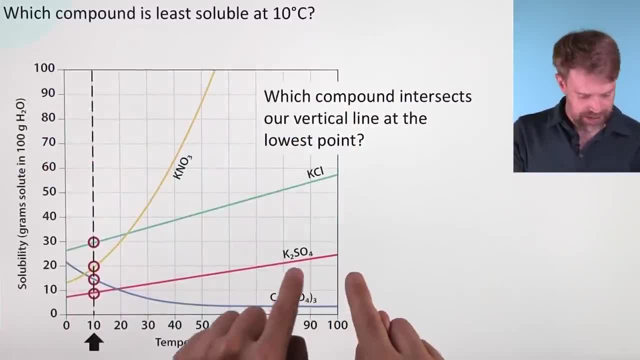 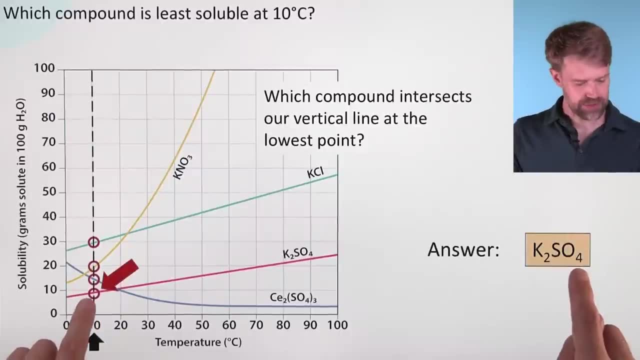 which of these lines intersects at the lowest point- and it looks like it's going to be this pink line here, which is K2SO4, potassium sulfate, and there's our answer. When you're doing problems like this, you always wanna make sure that you're paying attention. 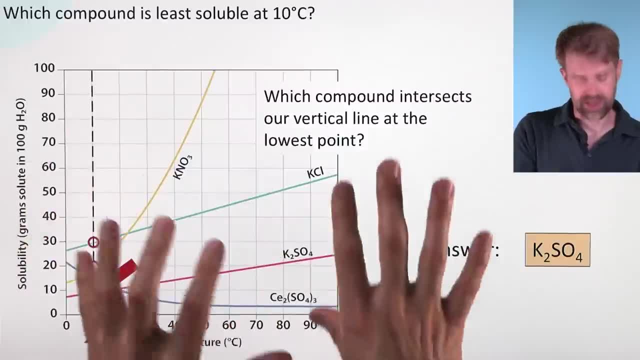 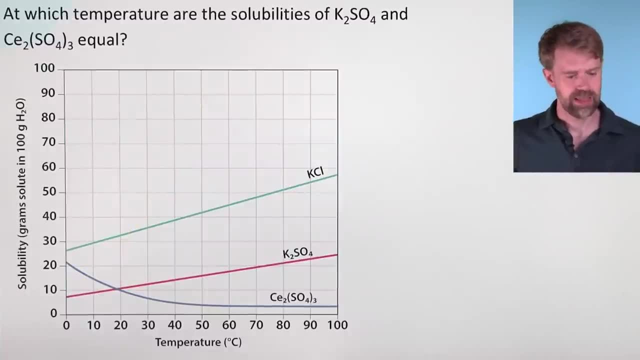 to the specific line. It can get a little bit tricky, believe it or not, to kinda keep them separate. so just make sure that the chemical that you find is associated with a line that you're looking at. Which temperature are the solubilities of K2SO4? 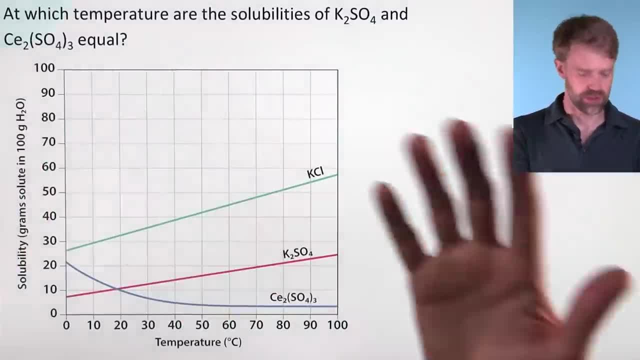 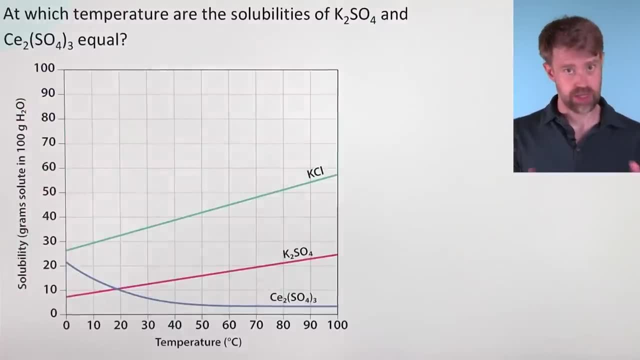 and CE2SO43, cerium sulfate equal. Okay, we're looking for where these two have equal solubilities. okay, Since solubility is plotted on the Y-axis, we wanna find the point where these two lines for these two chemicals have the same Y value. 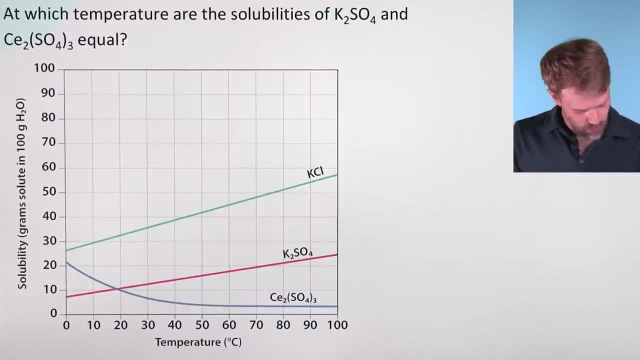 In other words, where they intersect- and that's gonna be right here- they have the same Y value. this point here Let's go straight down to the X-axis, which tells us temperature. you have to do some estimation. Let's say it's about 18 degrees. 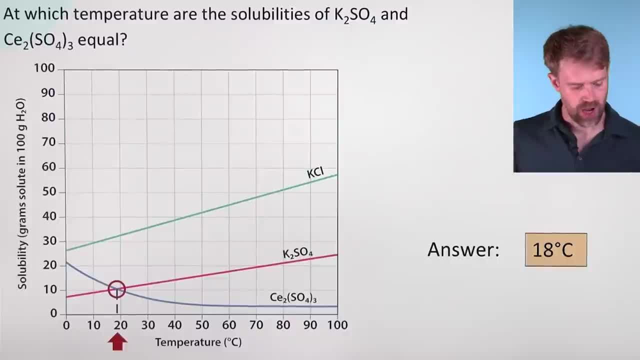 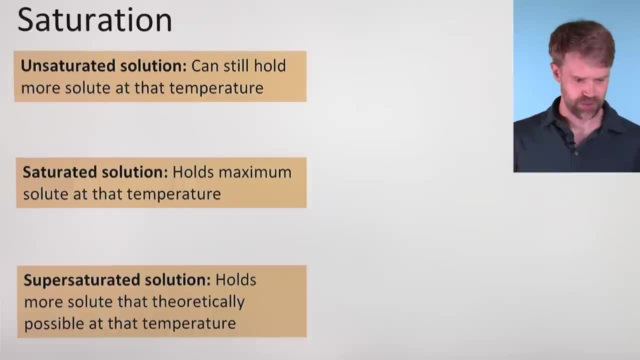 where they have the same solubility, where we see this intersection of the two solubility curves. Okay, now let's move on to a different type of solubility curve problem. We're gonna shift gears a little bit and we're gonna talk about saturation. 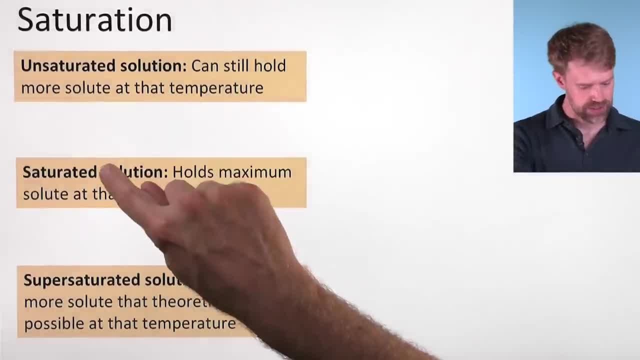 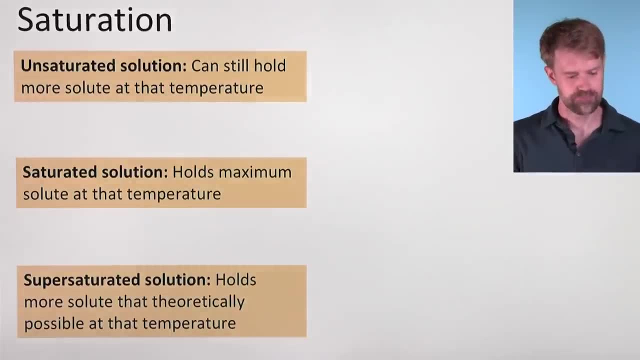 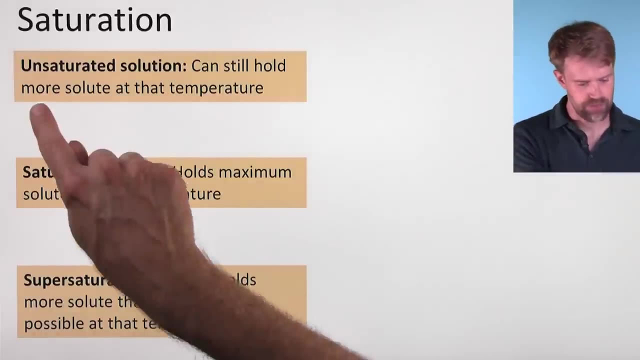 We're gonna look at some solubility problems that involve unsaturated, saturated and supersaturated solutions, But first let's quickly review these concepts. okay, An unsaturated solution is a solution that can still hold more solute at that temperature. 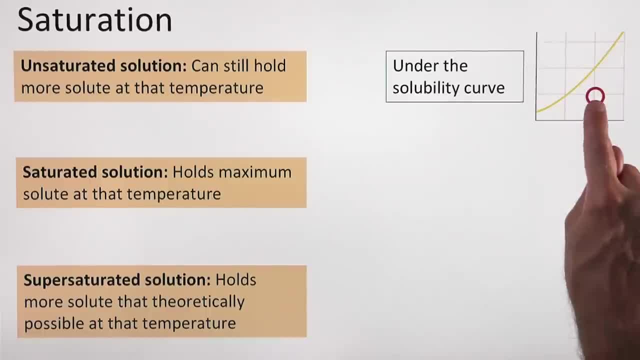 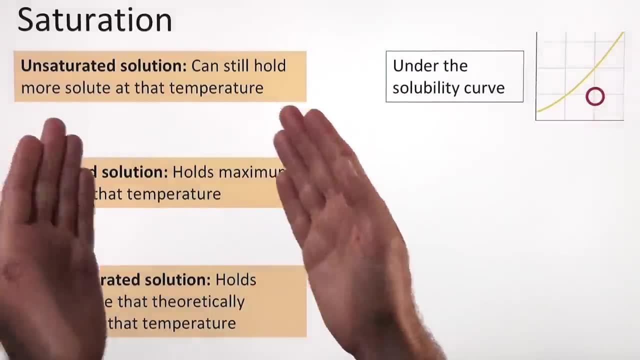 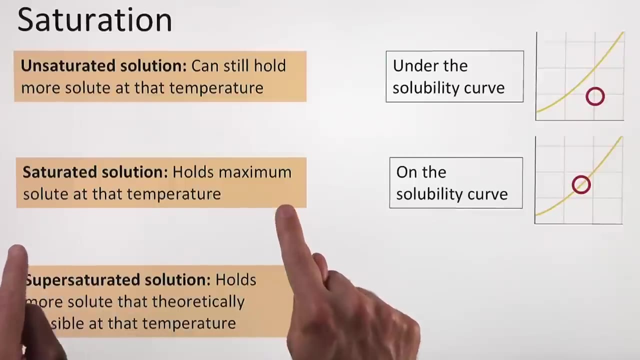 The amount of solute in an unsaturated solution would fall under the solubility curve because it's not yet at the maximum. This type of solution can still hold more solute Now. a saturated solution holds the maximum amount of solute at that temperature. 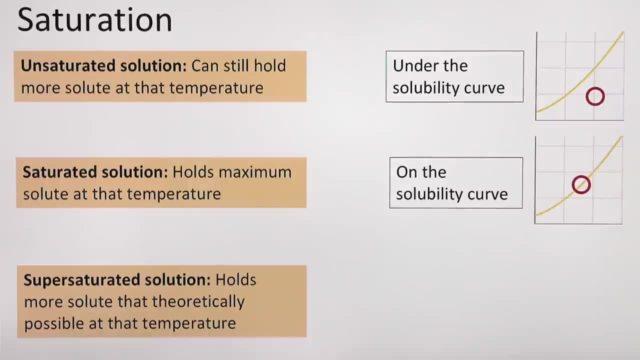 So if we plot the amount of solute in a saturated solution, it's gonna end up right on the solubility curve, which represents the maximum amount of solute at that temperature. And finally, a supersaturated solution holds more solute than is theoretically possible at that temperature. 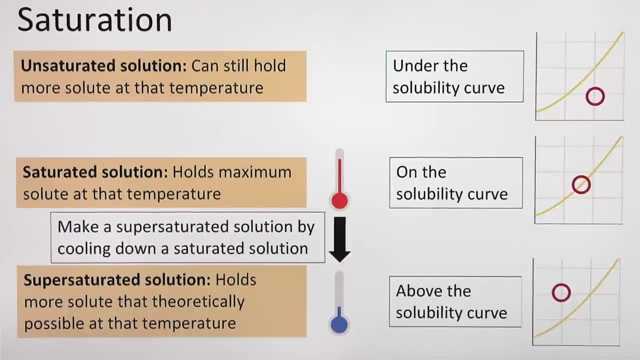 You usually make a supersaturated solution by cooling down a saturated solution and being careful not to disturb it. The amount of solute here would be above the solubility curve, because in a supersaturated solution we have an amount of solute that is temporarily greater. 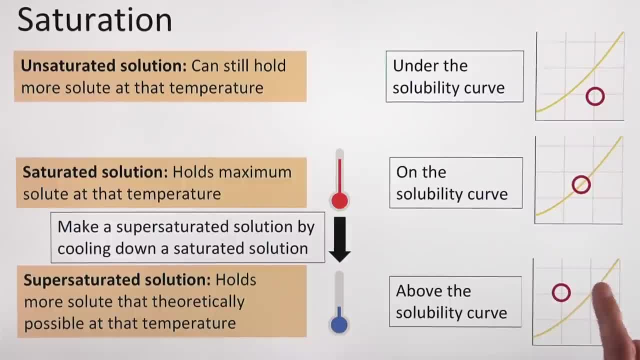 than what the maximum usually is. Okay, so the amount of solute here is going to be above the theoretical maximum. Now, if you're rusty on these concepts, you can check out a video where I focus just on this. but this is the amount of review. 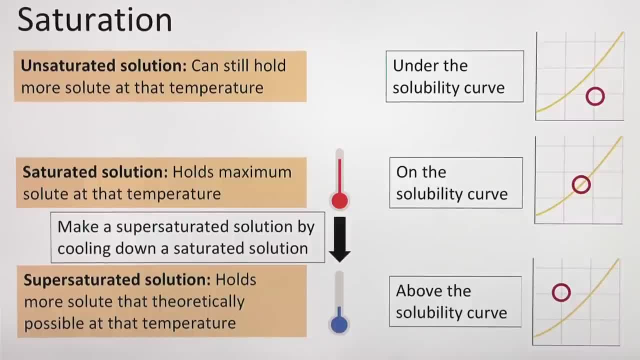 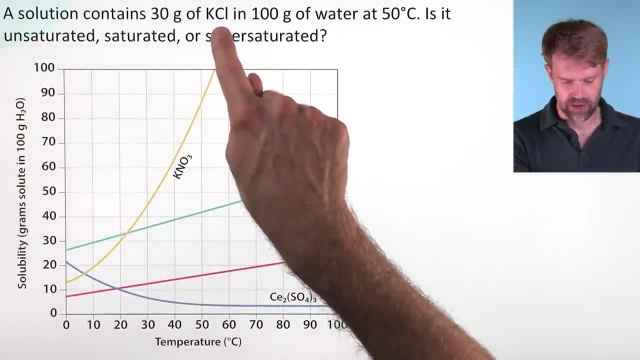 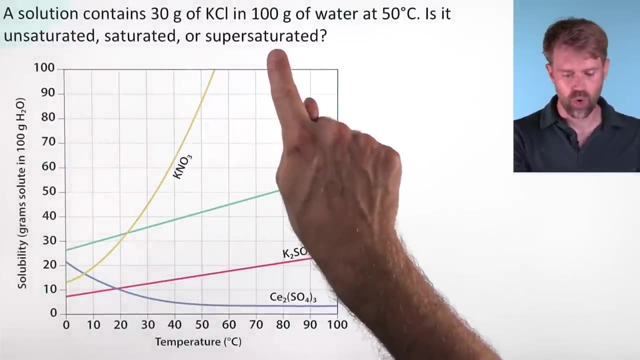 that we're gonna do for this video, which will allow us to tackle these next questions. A solution contains 30 grams of KCl in 100 grams of water at 50 degrees. Is it unsaturated, saturated or supersaturated? Okay, 30 grams in 100 grams of water. 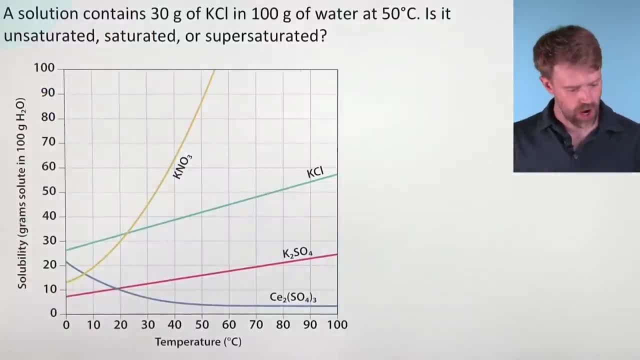 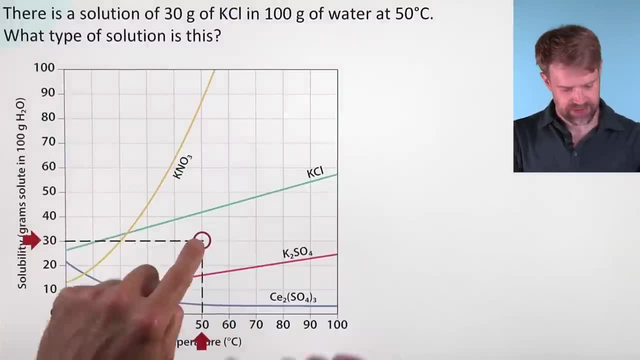 at 50 degrees. First, let's find this point on the graph. Okay, there's a solubility, There is the temperature. We'll head up and find the intersection point. Okay, there's the intersection point. and now we're interested in KCl, potassium chloride. 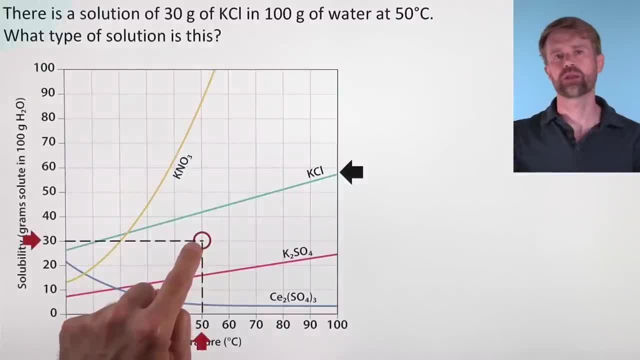 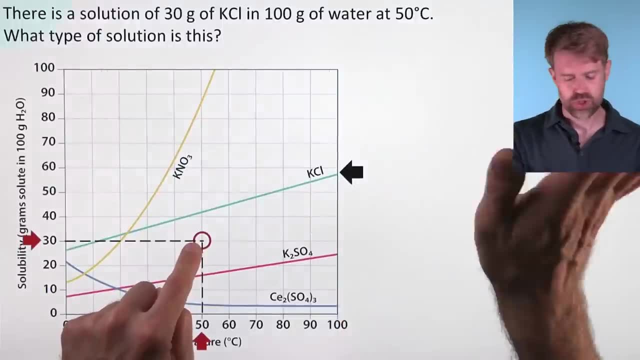 so we wanna pay attention to this line. We don't wanna worry about any of the other lines. When you're doing problems like this, make sure that you're looking at the right line for the chemical that you're being asked about. Super common mistake. so we're paying attention. 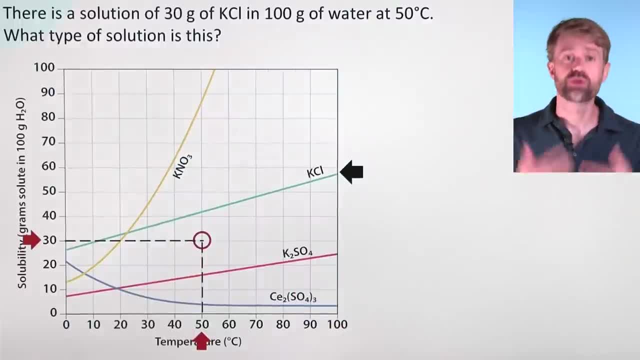 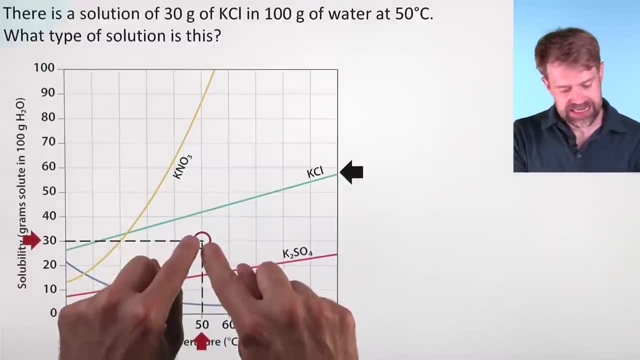 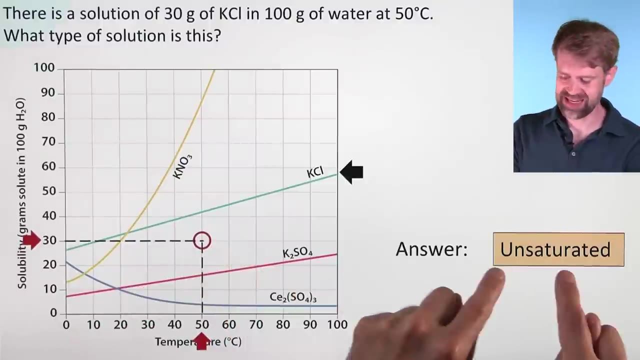 really to just this line right now. So the question that we wanna ask is: where is this point in relation to the line Right now? it's beneath this line. It's lower than the maximum, so that means that this point represents the amount of solute in an unsaturated solution. 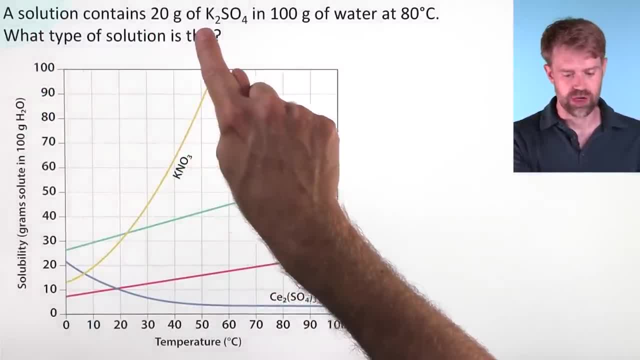 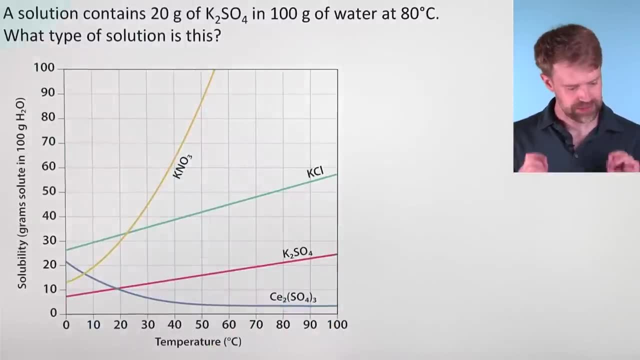 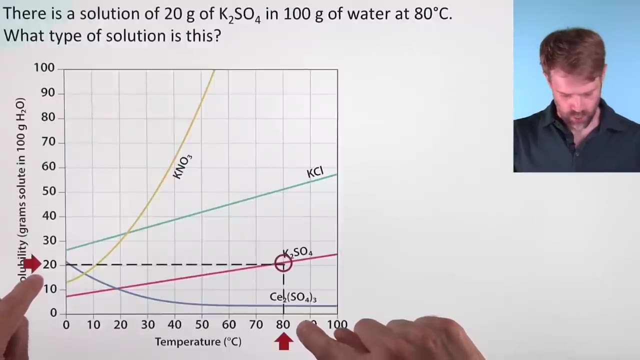 Here's another. A solution contains 20 grams of K2SO4 in 100 grams of water at 80 degrees Celsius. What type of solution is this? Okay, let's find these two points: 20 grams, 80 degrees Celsius. 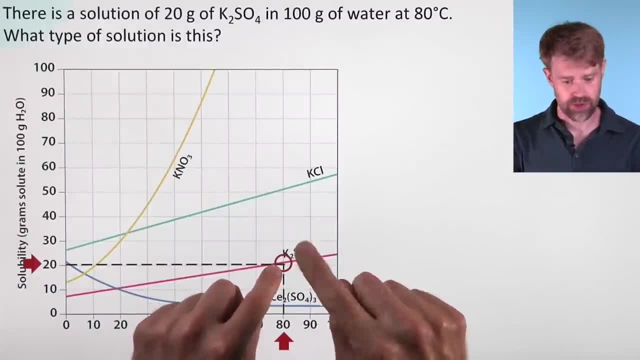 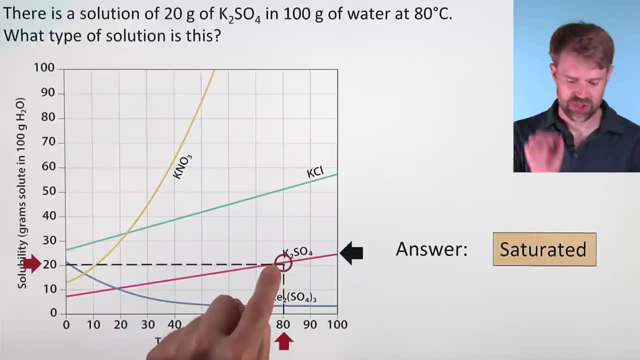 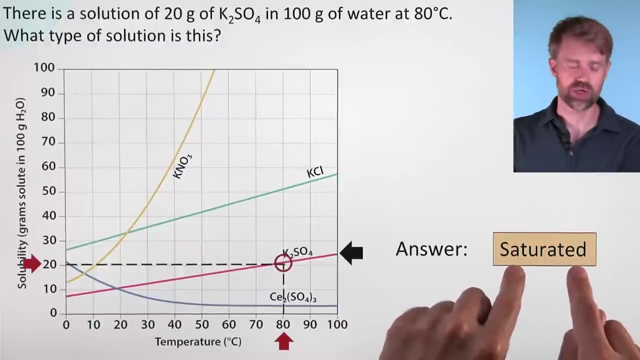 We find where they intersect. What's the solute that we're paying attention to here? It is K2SO4, it's this line. here The point hits right on the line itself. It represents the maximum, so it tells us that we're talking about a saturated solution. 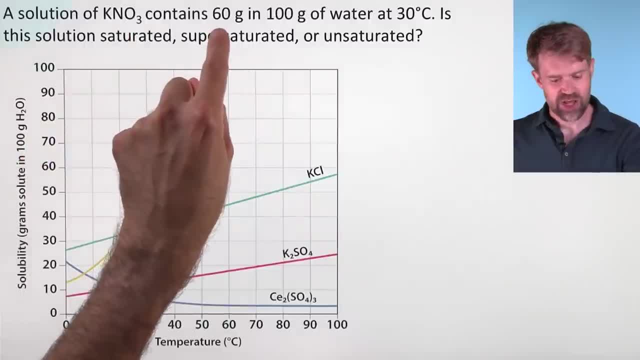 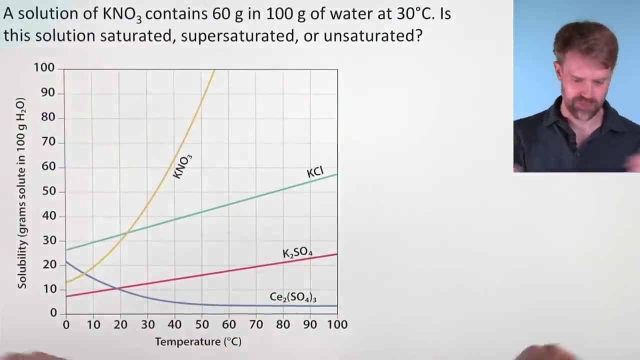 One more: A solution of KNO3 contains 60 grams and 100 grams of water at 30 degrees Celsius, Saturated, unsaturated, saturated, super saturated, unsaturated. You probably get the idea here. Here's the solubility. 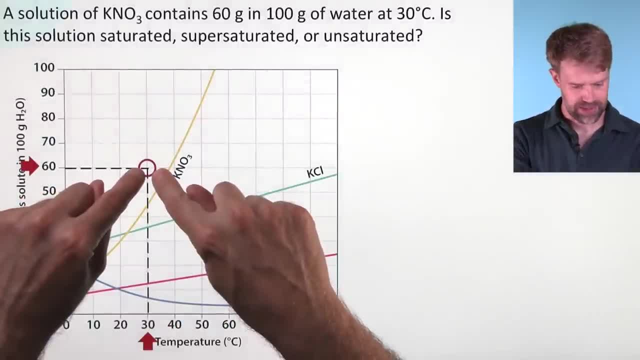 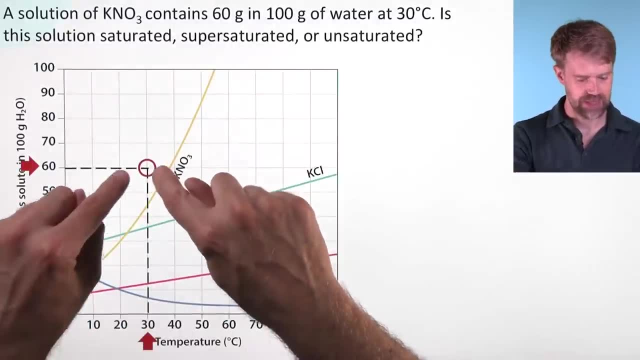 Here's the temperature. Let's see where they intersect. Right here We're paying attention to potassium nitrate, so we wanna look at this point in relation to this curve. As you can see, it is above this curve, so it represents a value that is greater than the theoretical. 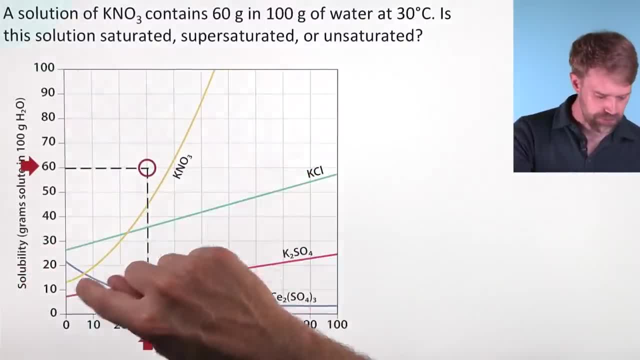 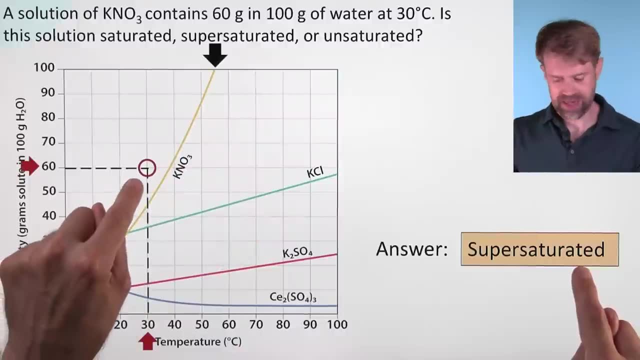 value of KNO3.. This is what I call solubility maximum of this curve right here, which means that since we're above the maximum temporarily, we're looking at a super saturated solution. Okay, now let's try a few final questions. 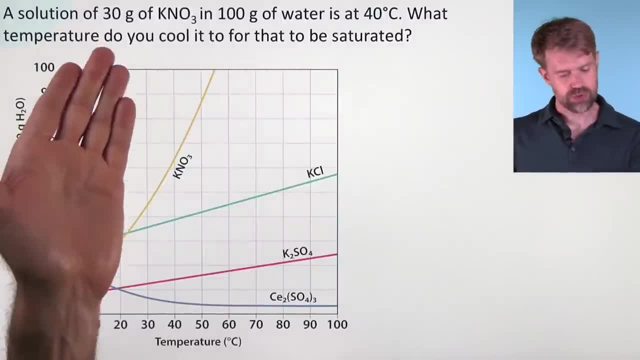 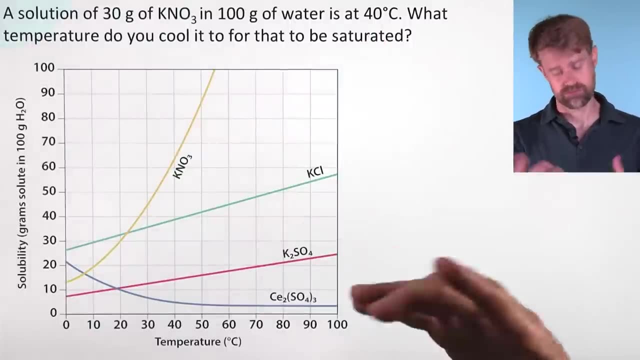 that have slightly different formats. A solution of 30 grams of potassium nitrate in 100 grams of water is at 40 degrees Celsius. Okay, what temperature do you cool it to for that to be saturated? Okay, so first we'll start out by finding the point. 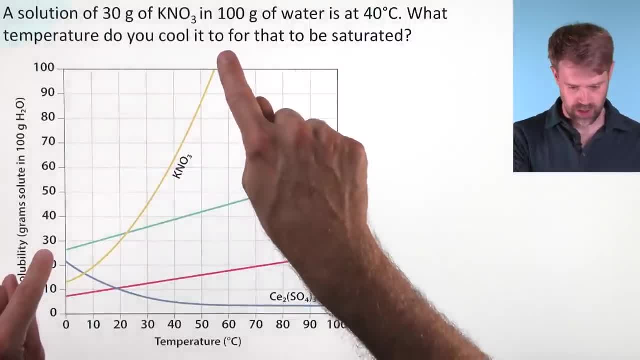 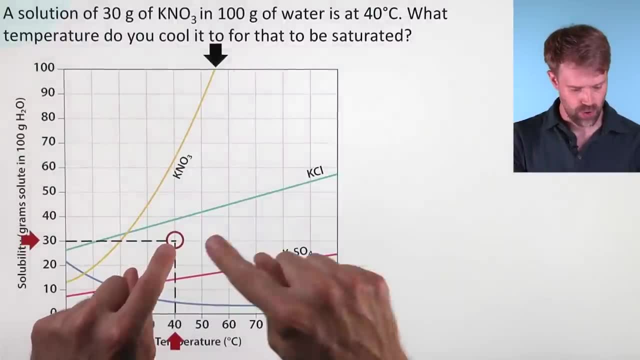 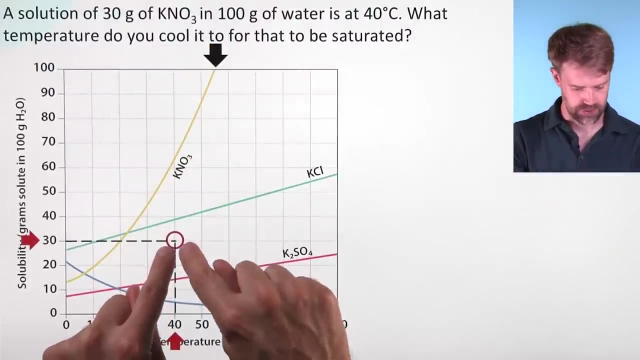 that we're describing here. Okay, 30 grams per 100 grams of water at 40 degrees Celsius. Those are our two points. We intersect right there. Okay, now we're looking at this point in relation to the curve that gives us a solubility for potassium nitrate. 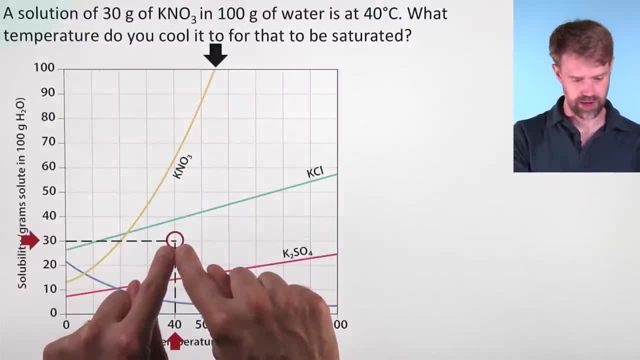 Okay, this is an unsaturated solution right now, because it's below the line. Okay, Now we want to find out: what temperature do we cool this to for it to be saturated? Well, if it's going to be saturated, it's going to be right on the line. 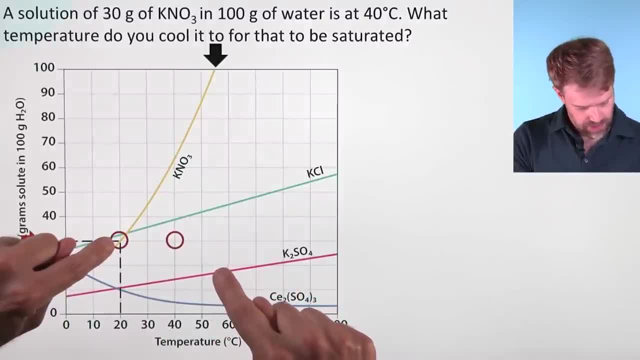 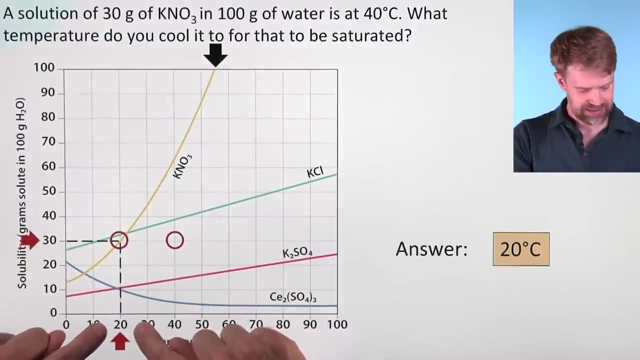 So we want to cool it down to this point here. Bam, right there. Let's look at what temperature that corresponds to. We go down to the x-axis and that looks to be just about 20 degrees Celsius. This will be a saturated solution. 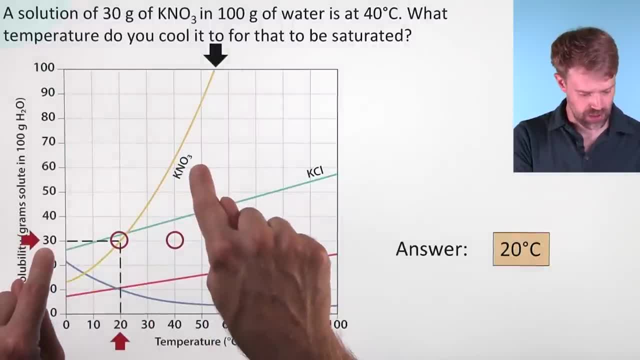 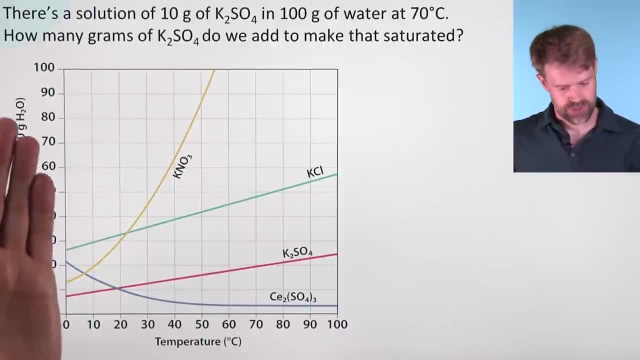 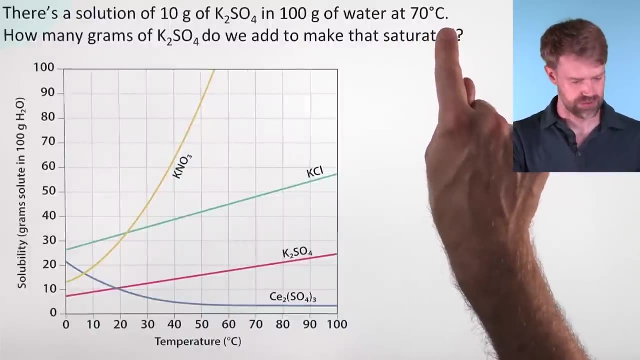 with 30 grams of potassium nitrate dissolved in 100 grams of water 20 degrees Celsius. Here's a different type of question. There's a solution of 10 grams of K2SO4 in 100 grams of water at 70 degrees Celsius. 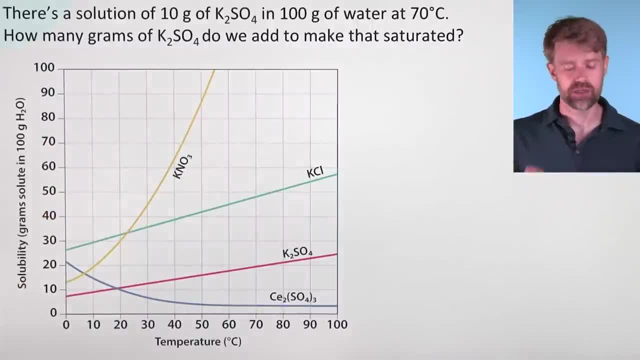 How many grams of K2SO4 do we add to make that saturated? Okay, let's find this point on our graph: 10 grams per 100 grams of water, 70 degrees Celsius. right there, Okay, K2SO4, we're going to be paying attention to this line. 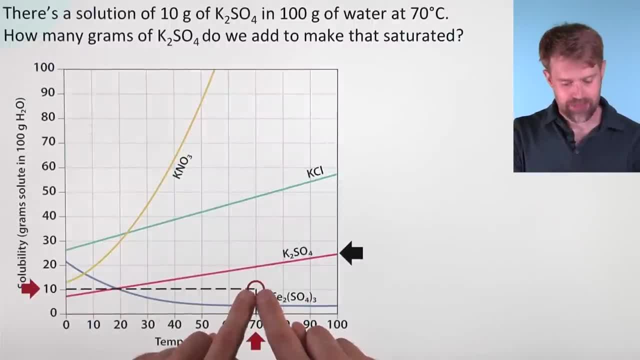 Okay, We're underneath it, so it's unsaturated. right now, How many grams do we need to add to make that saturated? Okay? well, if we want a saturated solution, we're going to want to be right on that line. 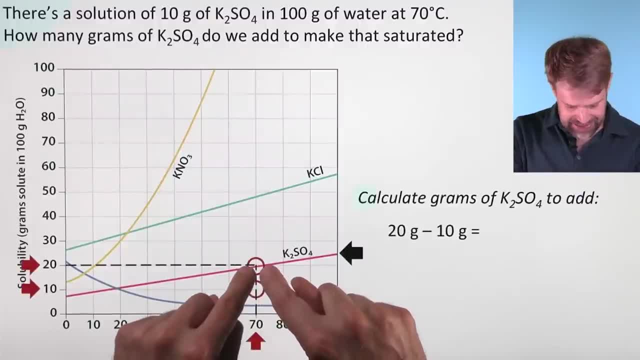 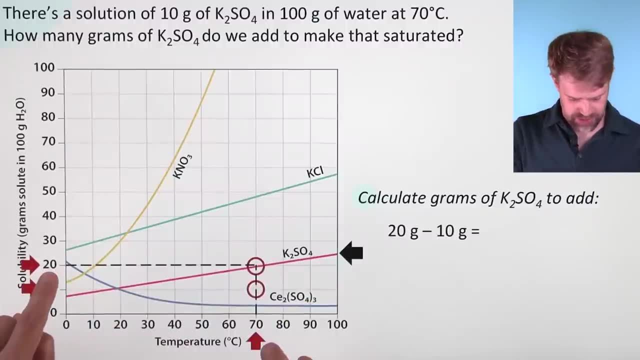 So we're going to want to be at 70 degrees and this value on the y-axis, which is going to be 20 grams, All right, 20 grams and 70 degrees would be a saturated solution. So 20 grams. 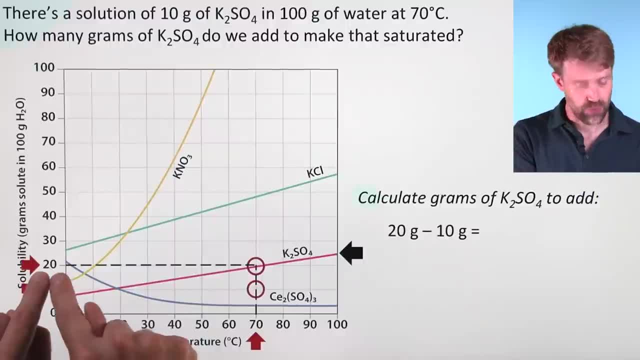 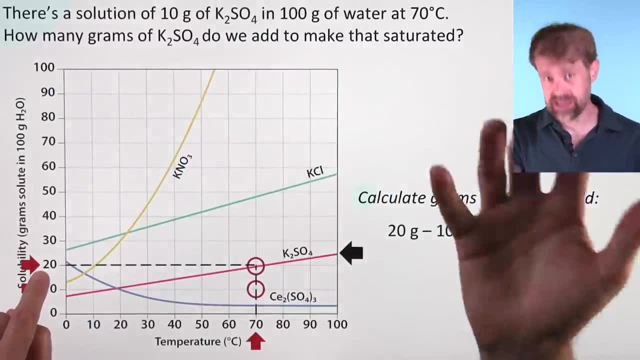 20 grams is what we would need for it to be saturated. but we're asked: how many grams do we need to add? right, It's not how many grams is in a saturated solution- how many grams do we need to add? So 20 grams for the saturated solution. 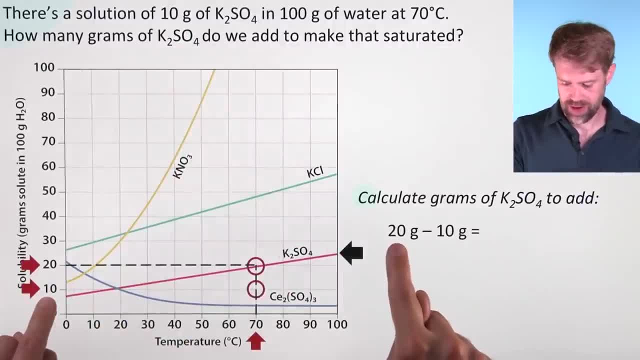 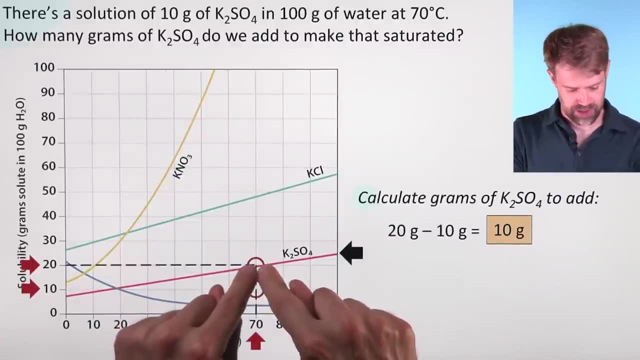 minus. we already had 10 grams. 20 grams minus 10 grams equals 10 grams. We need to add 10 grams to this solution. to bring it up here, to put 20 grams, 20 grams, 20 degrees, 20 grams in 100 grams of water at 70 degrees Celsius. 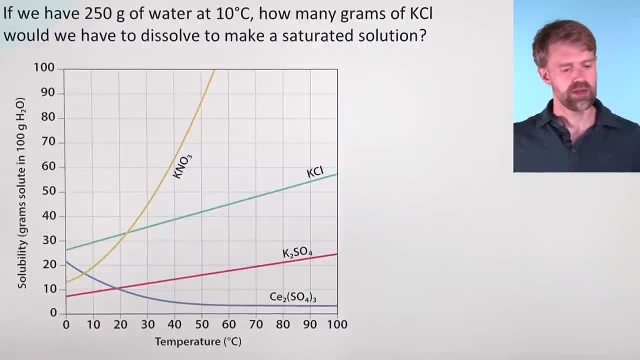 to make a saturated solution. These last two problems will involve some math and conversion factors. So far, we've talked about everything in 100 grams of water, because that's what our y-axis has corresponded to. okay, These final two questions are going to talk about. 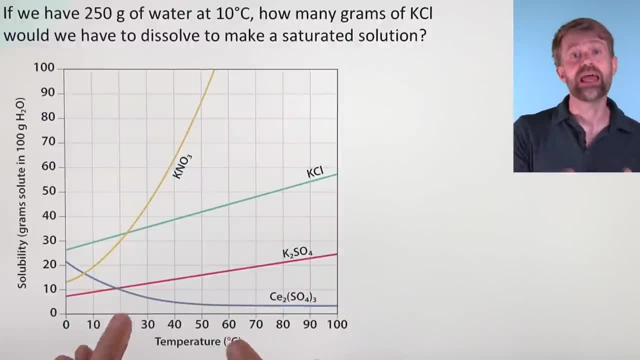 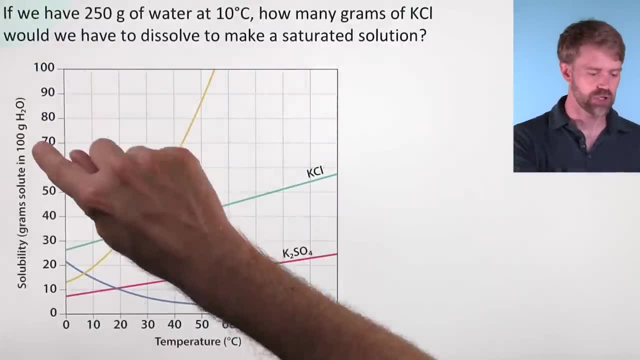 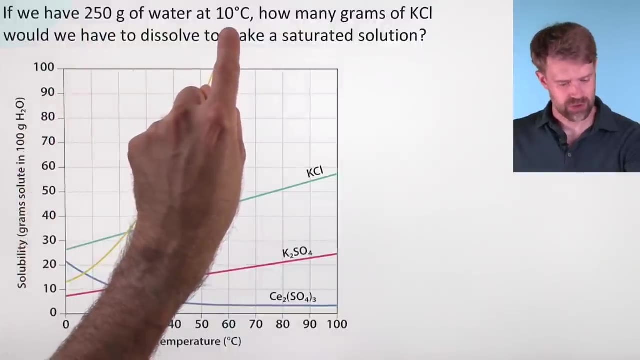 different amounts of solute dissolved in an amount of solvent that is not 100 grams. okay, So we'll have to use some conversion factors to go from 100 grams of solvent to a different amount. okay, If we have 250 grams of water at 10 degrees Celsius? 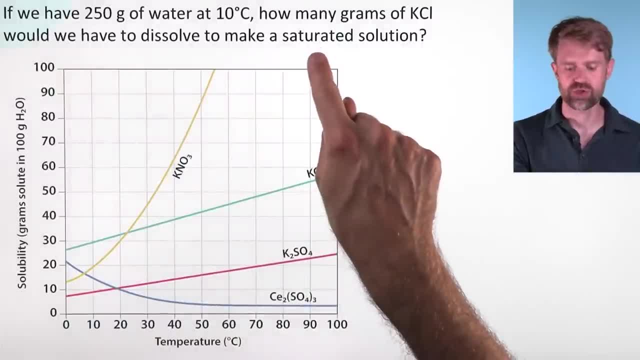 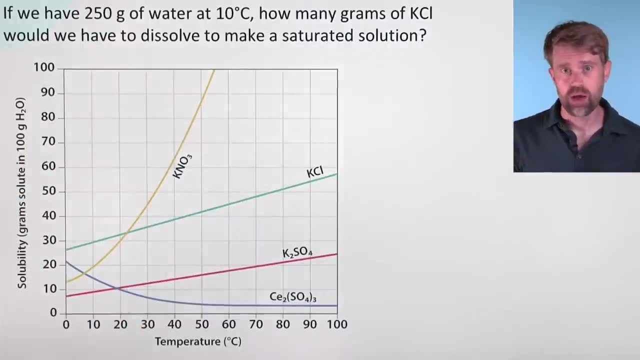 how many grams of KCl would we have to dissolve to make a saturated solution? Okay, here we're talking about 250 grams of water, but let's start out by figuring out what a saturated solution would look like in 100.. 100 grams of water, okay. 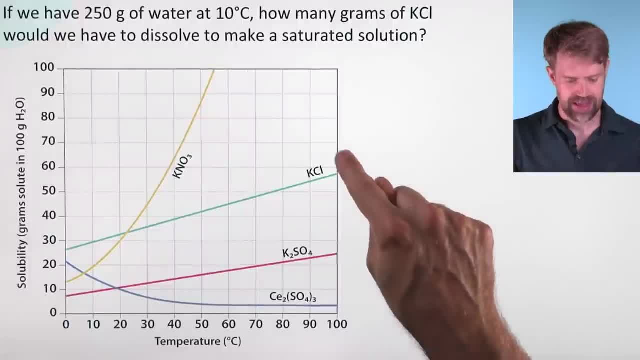 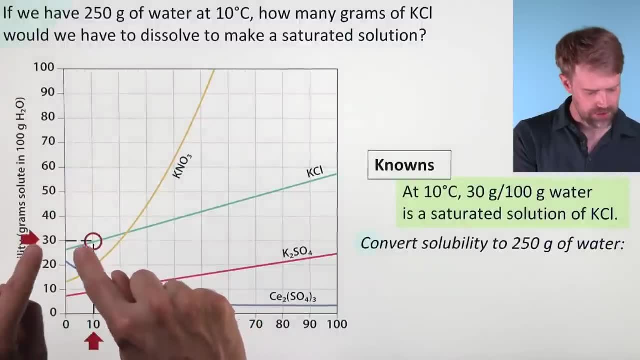 So we're talking about KCl. that's gonna be this line here: 10 degrees Celsius. okay, Let's find 10 degrees Celsius, go up to the line and go across here: 30 grams of KCl in 100 grams of water. 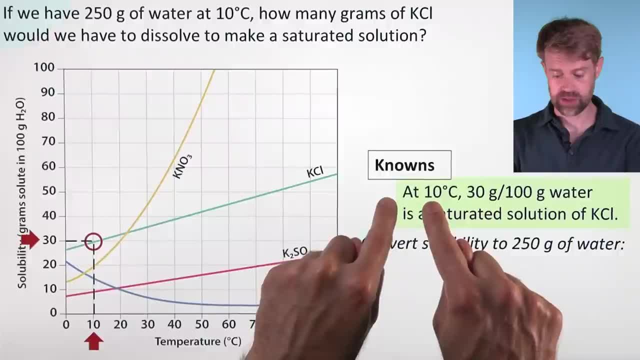 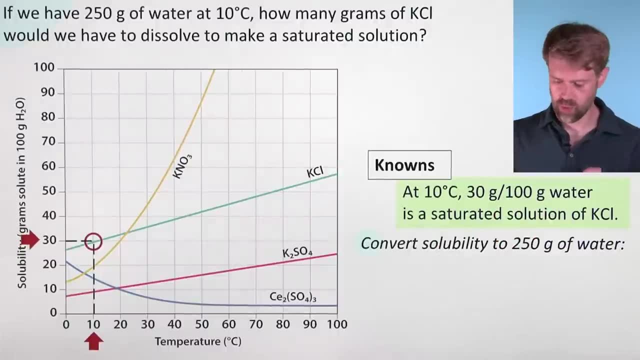 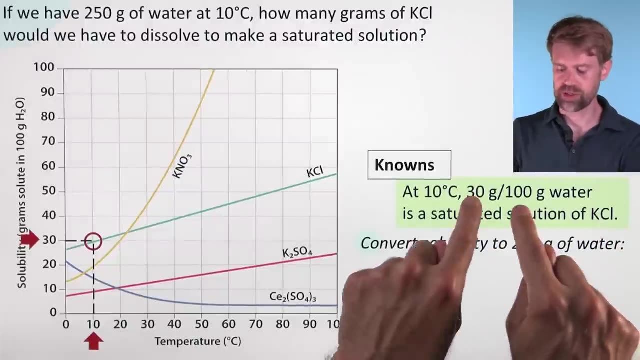 is a saturated solution. okay, 10 degrees, 30 grams per 100 grams of water. But this tells us how much is gonna dissolve in 100 grams of water. We need to convert it to 250 grams of water So we can use the solubility as a conversion factor. 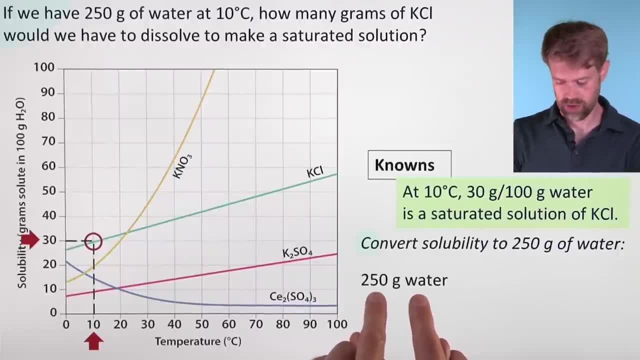 We start out with 250 grams of water and we multiply it by the solubility expressed as a conversion factor. okay, 30 grams KCl per 100 grams of water- Now, grams of water- is gonna cancel out. We multiply this by this.